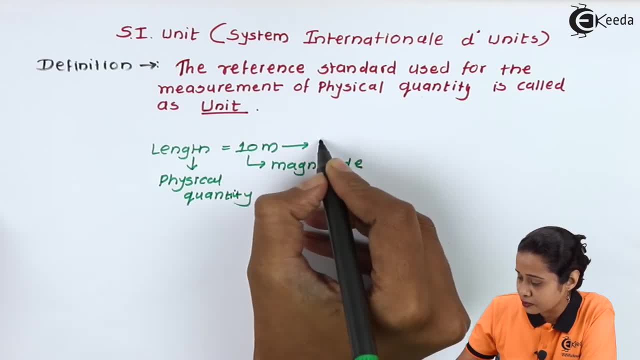 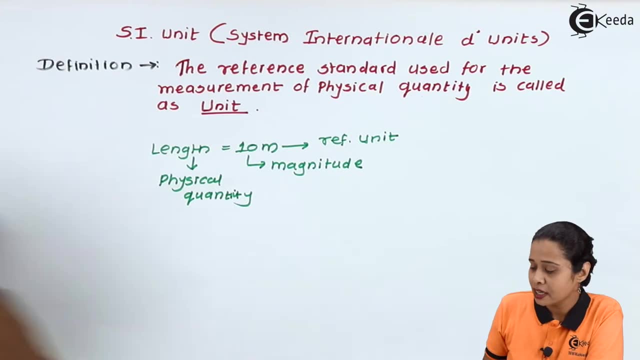 So we can say: length is 10th meter. So we can say length is 10th meter. So we can say length is a standard or reference unit. Means in simple way we can say: the length is 10 times of a standard unit, that is meters. So in: 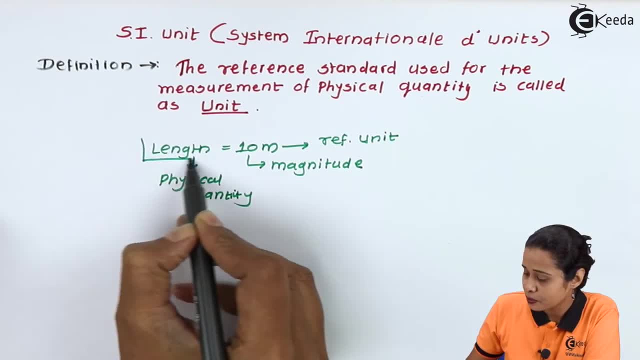 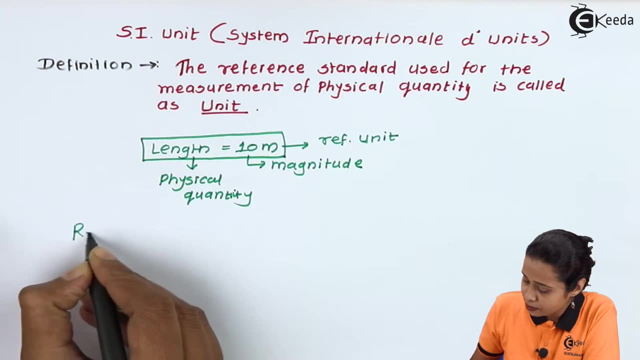 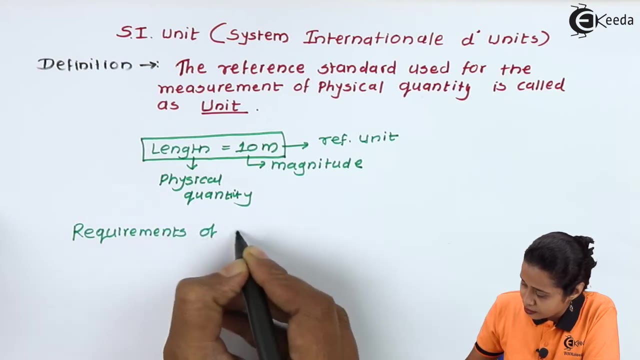 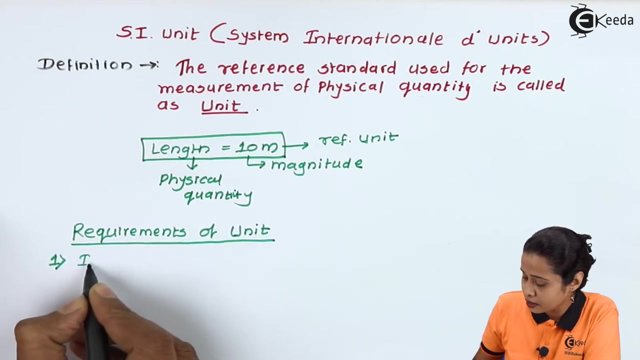 this way we can find out the units. Let us see what are the requirements of good units. So in simple way we can write down requirements of unit. The first requirement here is it should be well defined and common Means. unit should be well defined and common Means. we can easily use it. 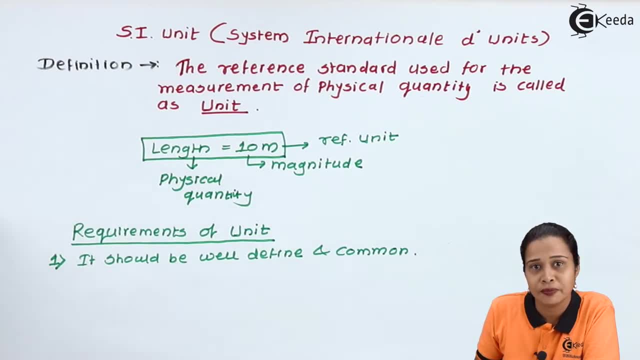 Suppose we want to take a vegetable for 1 kg, So kg that commonly we use. if you want to purchase a cloth we can say 5 meters of cloth. 10 meters of cloth meter is also very commonly we use. 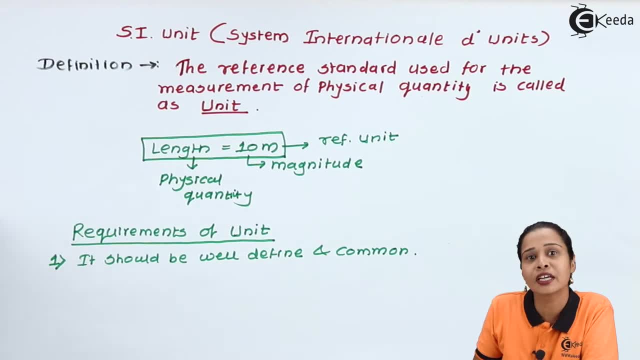 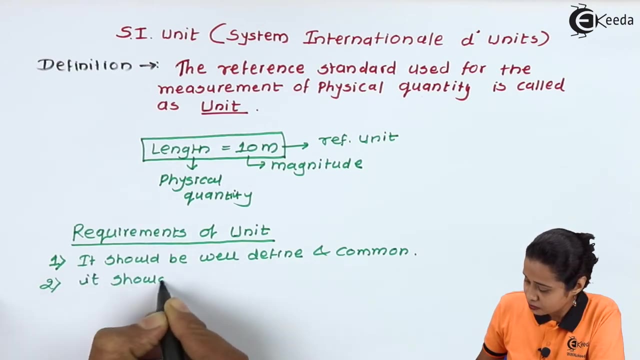 So it should be easily accessible, or we can say it is commonly used, So it should be well defined as well as common. Second requirement is it should be convenient. size Means unit should not be very large or it should not be very small. 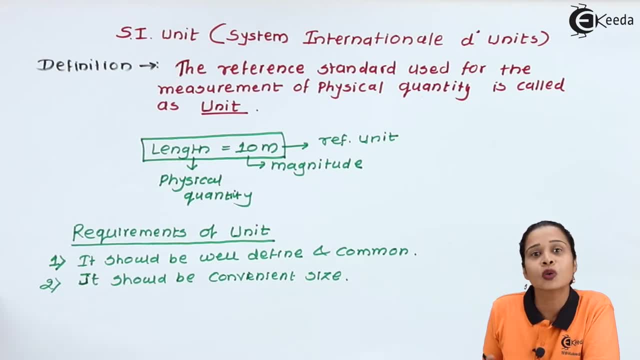 Means. if you want to purchase a vegetables, we will go to the shop and we will ask for 1 kg of tomato. But if your unit, if you are defining unit at the very large scale, means instead of kg you are defining basic unit as a ton, then you have to go to the shopkeeper. 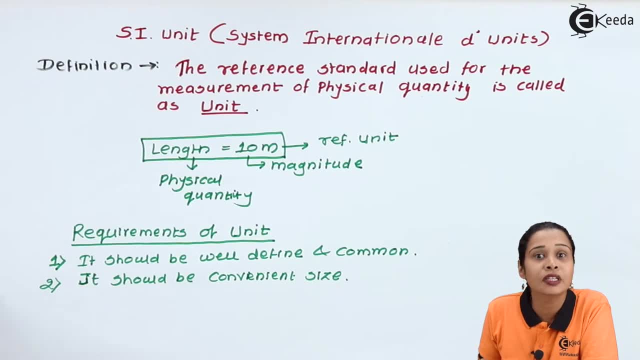 And you have to ask him, for I want 1 upon 1000 tons of tomato, So this is very difficult to explain. Actually it is equal to 1 kg, but that size is very large. That's why we required unit that should not be very high size and it should not be very less.